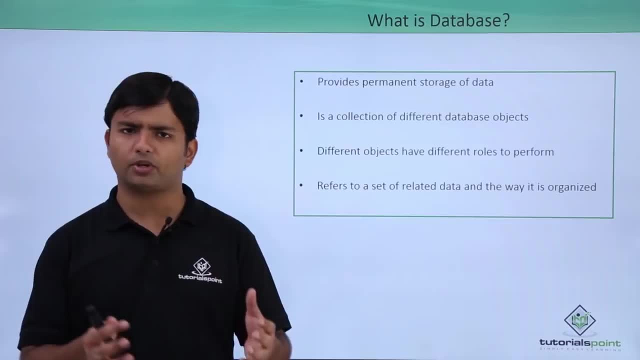 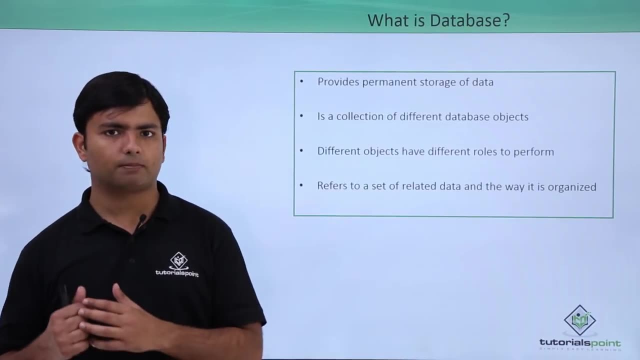 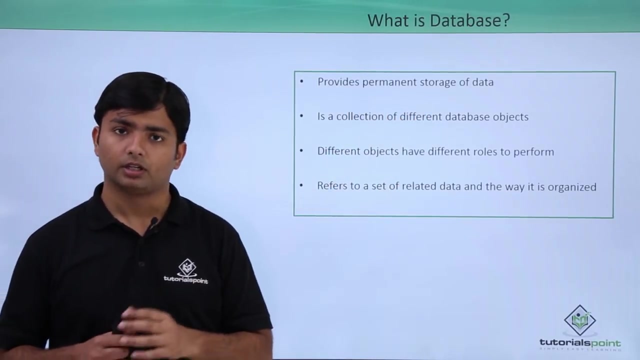 in which the user cannot make a direct interaction, because user generally makes the interaction with the user interfaces, ie the UI, maybe the web page, maybe the mobile application. you are dealing with database, so this database actually provides the permanent storage of the data. so when we talk, 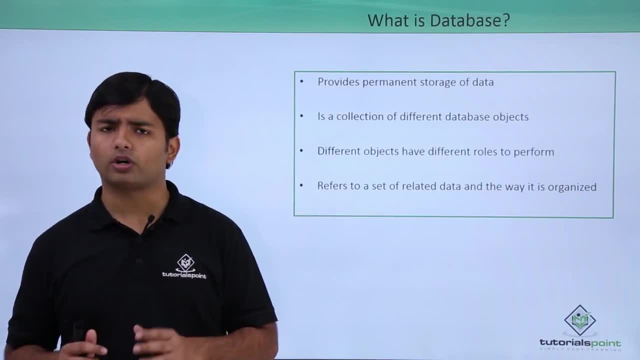 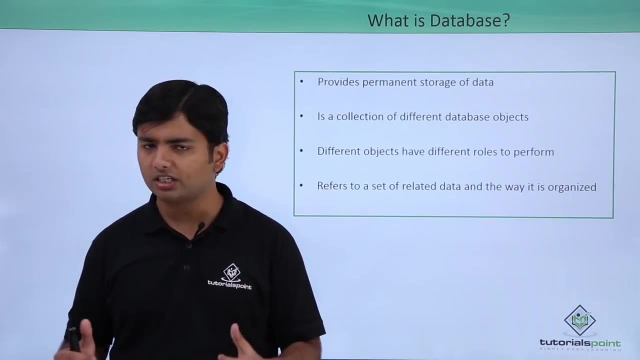 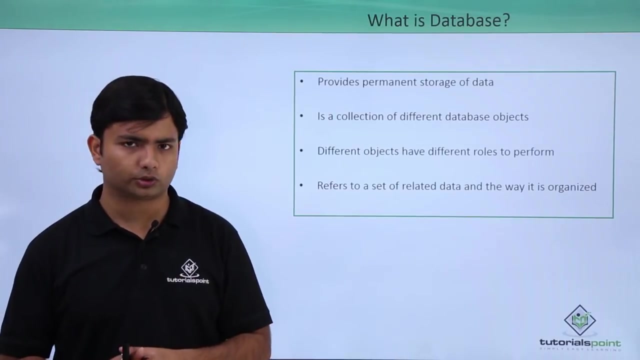 about storing the data. the data is actually stored in a tabular way and all the data is related to each other, for example, if i am talking about the database of a company like tutorials point. so here the tutorials and the writers who write those tutorials, the video tutorials, all are somewhere. 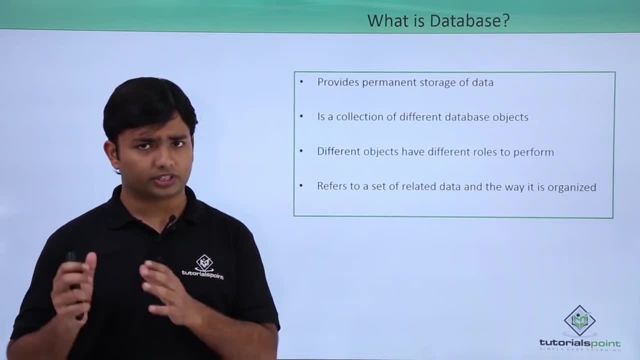 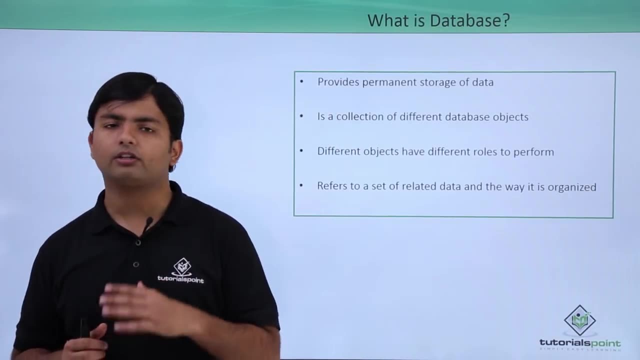 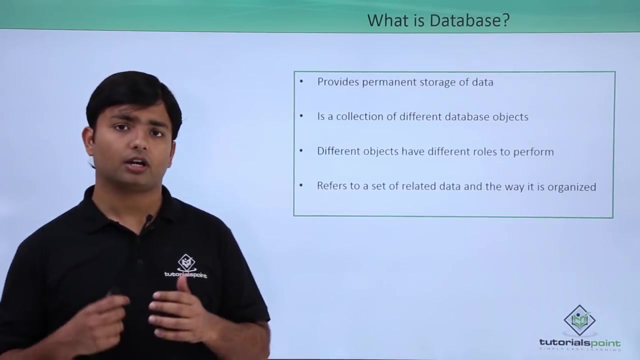 related to each other and will be stored. the data will be stored in the tabular way but in the database table is not the only thing which is stored, as it may have the number of different types of object for the different purposes. so, like here, i just talked about the tables we may get. 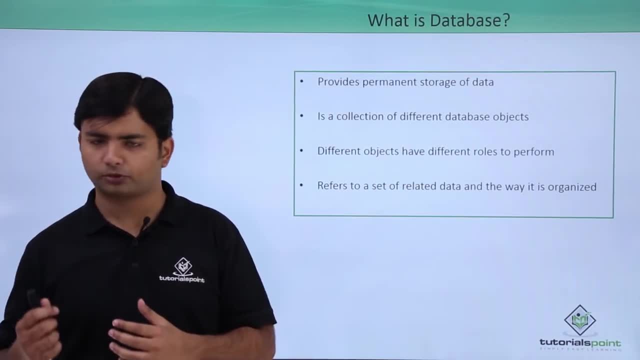 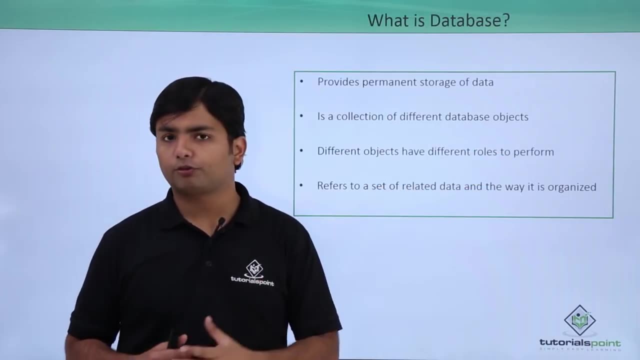 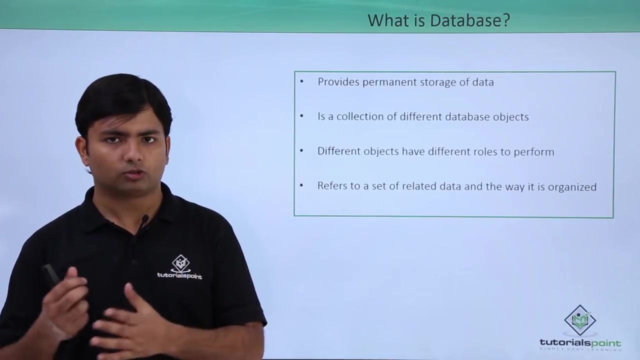 something like views, indexes, synonyms, procedures, functions, which you will find in this video tutorial. different objects have the different roles to perform. like table. goal is to store the data. similarly, if i talk about the views, it will be used to restrict the data. maybe if i if i talk about the triggers, it will do some validation or maybe some. 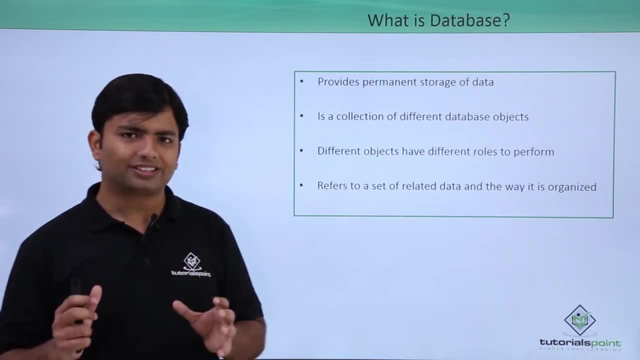 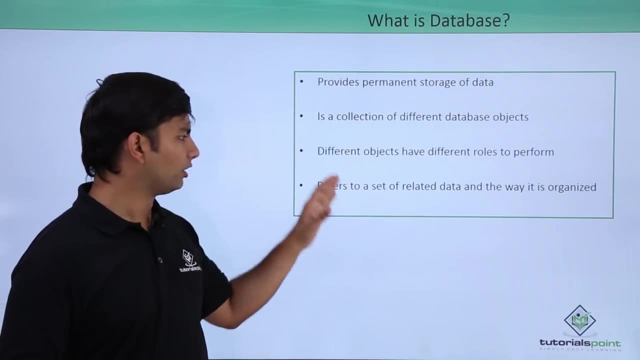 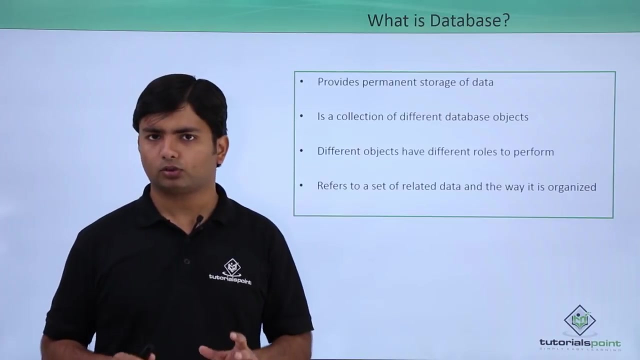 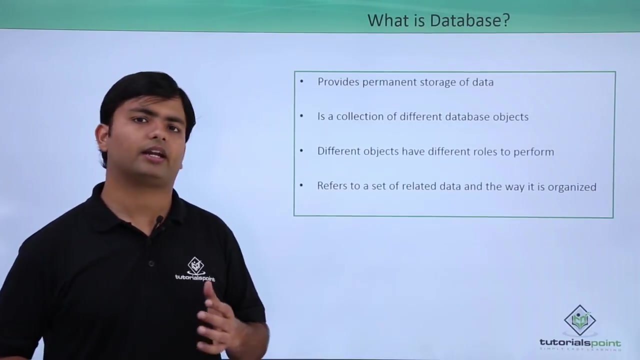 implicit, will take some implicit actions. so basically, each and every database objects have a different role to perform. so basically, in database it refers to the related set of data and the way it is organized. so once we have the database, obviously we should have something which will help us out to interact with the database and in that sense we will talk about 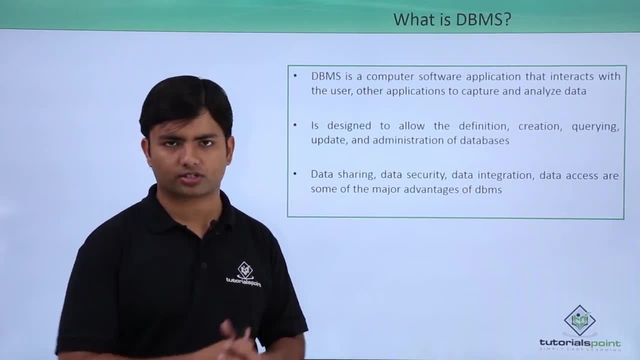 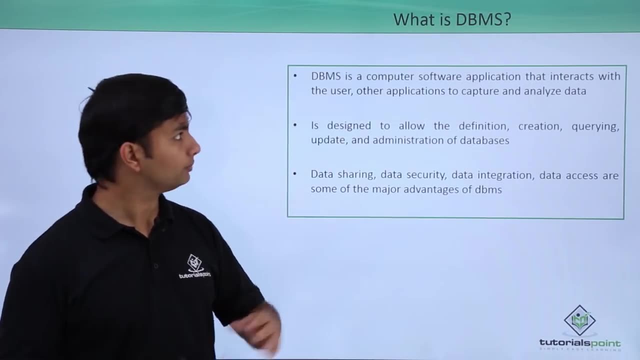 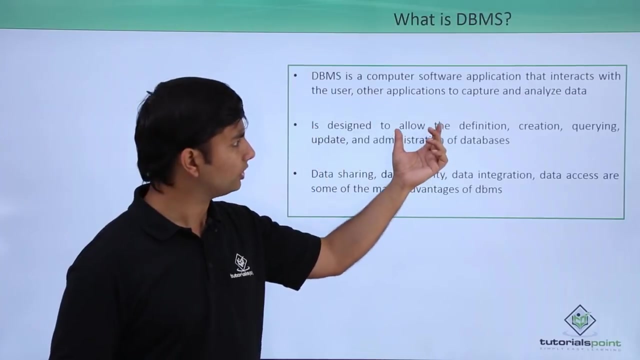 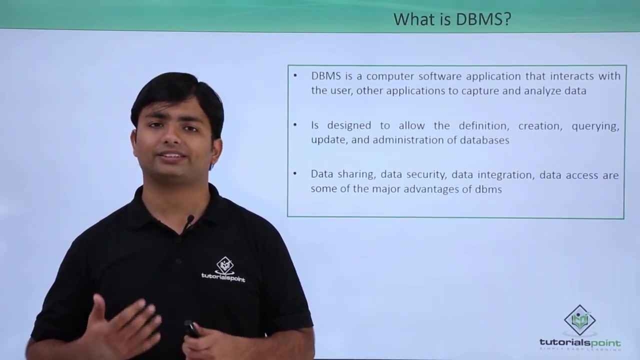 the dbms, that is, database management system. so database management system is basically a way to interact with the databases, as here. dbms is a computer software application that interacts with the user or other applications to capture and analyze data. for example, there is a database. i want to access the database directly. maybe if i am a dba i can sit on the database server can start. 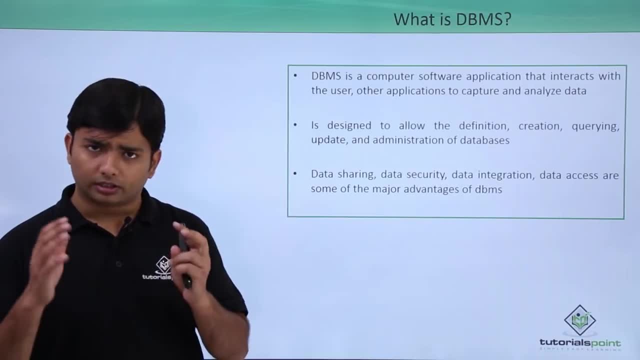 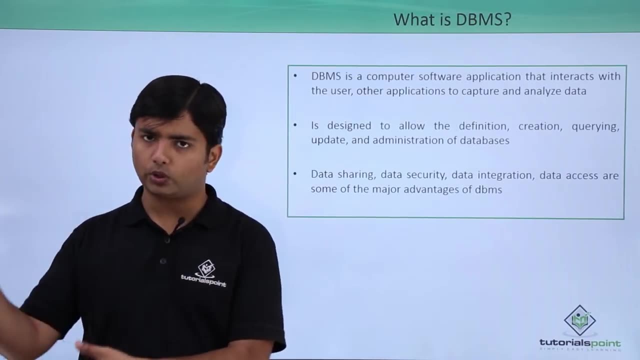 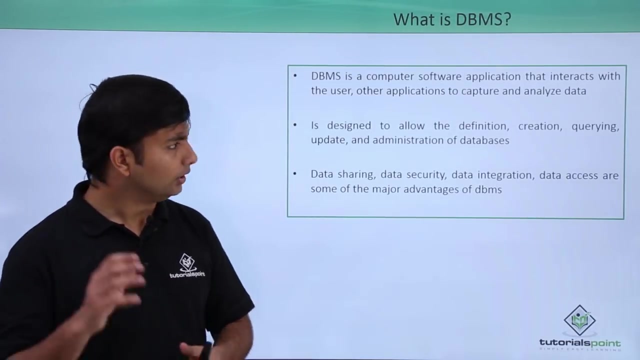 fetching the data directly, but generally what we do, this database would be accessed by some application like. i just give an example of facebook. the data is stored in the database, but that facebook application is actually retrieving the data from the database and then retrieving the information from the database. so this is all possible because of this. 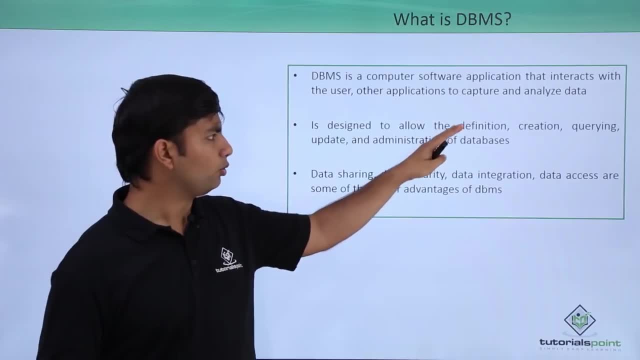 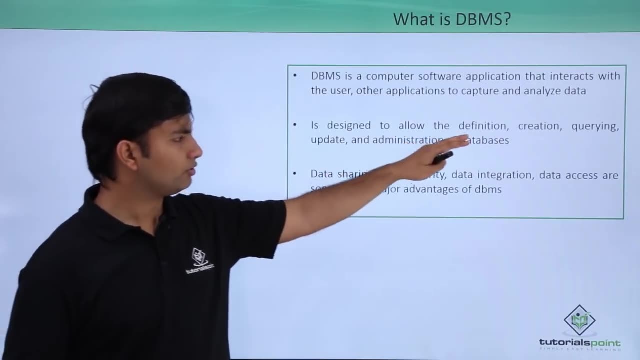 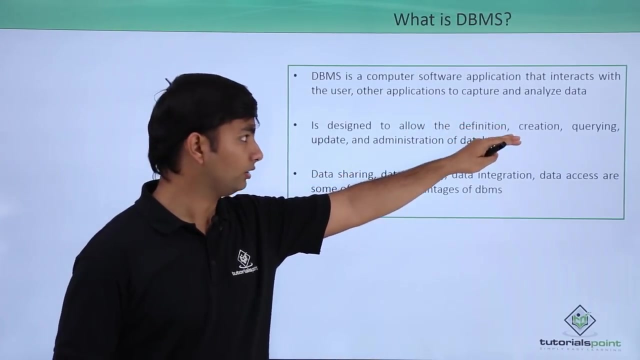 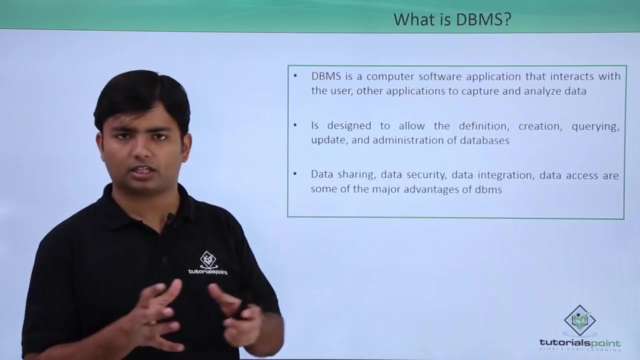 dbms. so this dbms is designed to allow the definition, creation, querying, update and administration of database. definition means if you want to create a new table or any database object, that is the creation, definition and and similarly, you can create the database objects. once you have created the database objects and you have stored the data, you can query the data, you can update the. 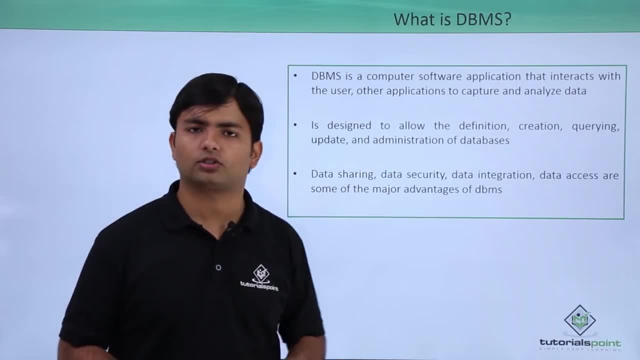 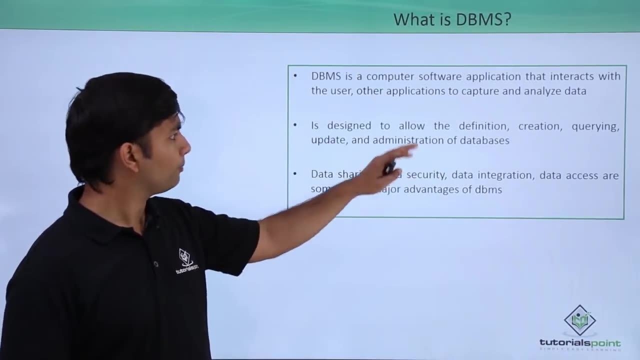 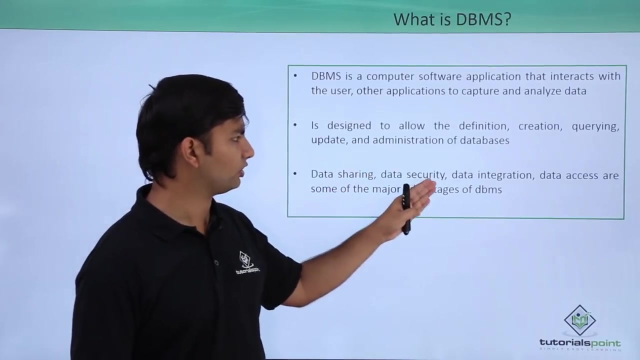 structure or the data and you can administer like you can pass some validations, you can set some privileges to the different set of users and all. so these are all can be possible because of this dbms. data sharing, data security, data integration, data access are some major advantages of data dbms. 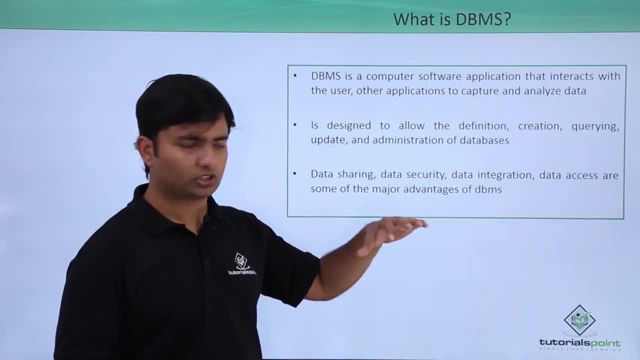 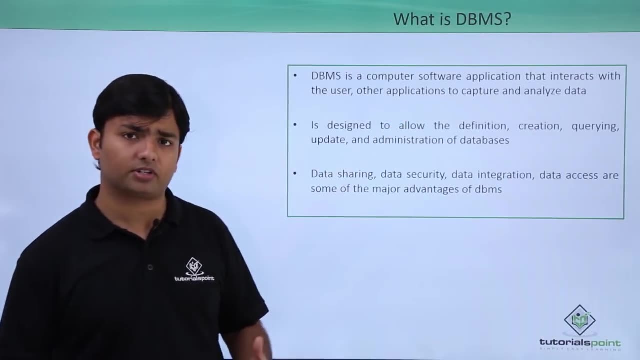 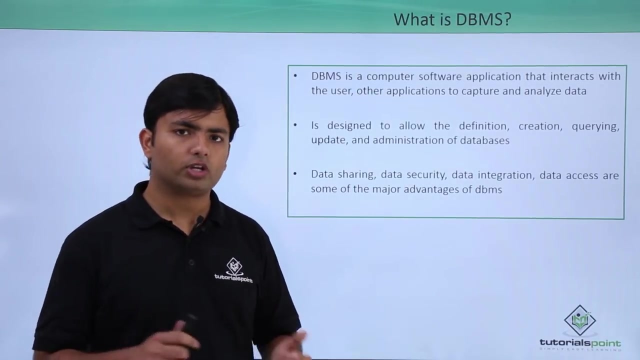 data sharing if you want to share your data secure, putting the security in data integration and accessing the data. so all that thing, those things can be done with the help of the dbms. but nowadays the dbms which we are working is our dbms, that is, relational database management system. 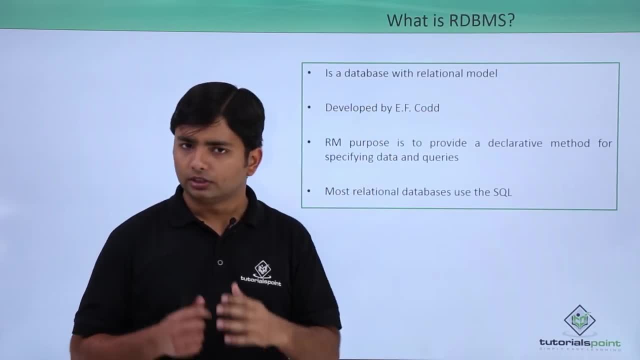 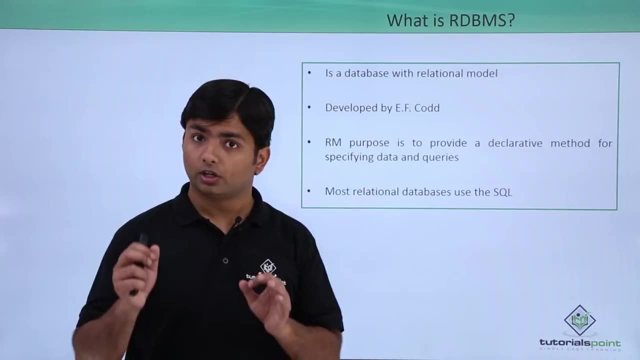 basically, this model is launched by dr ef cord. so basically, he wrote a new dbms database and the data in this dbms database is a database of all types and he crafted it for a few different issues in order to decorate within this dbms database and his 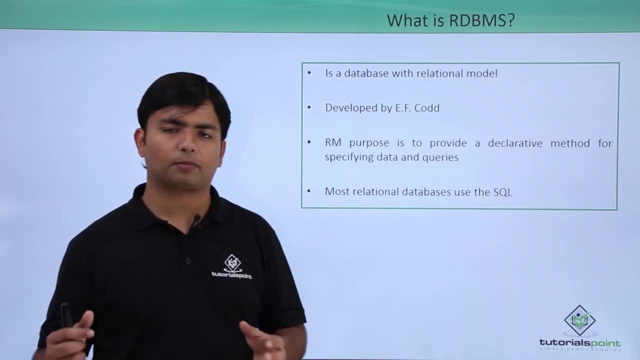 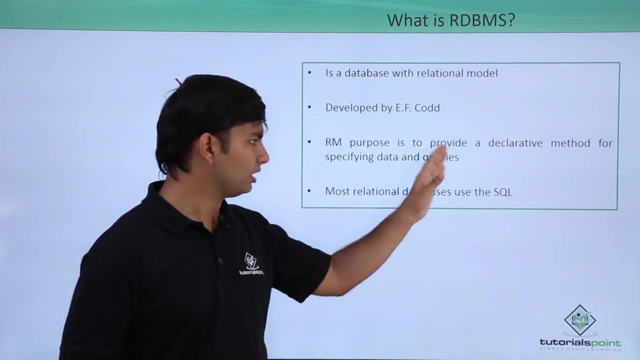 piece of work is that if you want to design a database that is related to your database, then you have to identify your database and how you want to manage it, and also you can initialize a database based on your database. right, so you can create a database using a database. 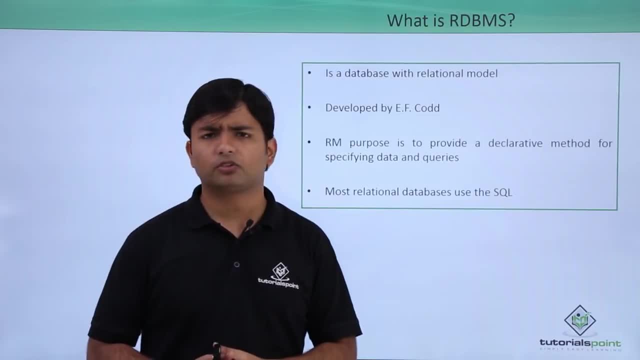 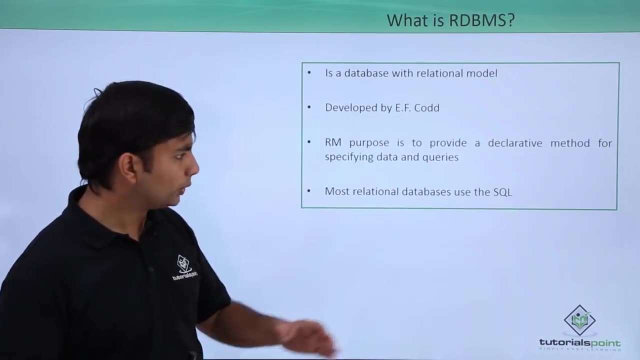 so here you are using a database, right? so basically, dbms is your database, your database, that is located in your database and it is your database. data sharing and the dbms Göring and the other two are important. use the SQL as the query language, SQL, which stands for structured query. 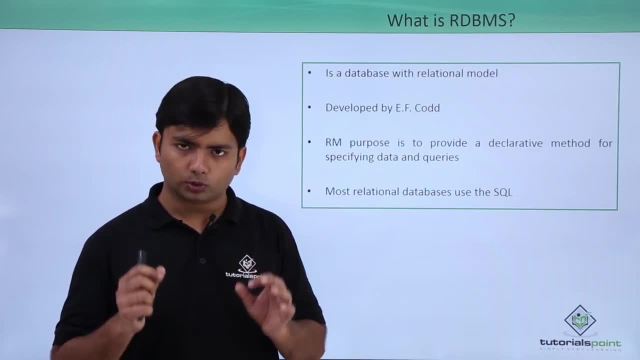 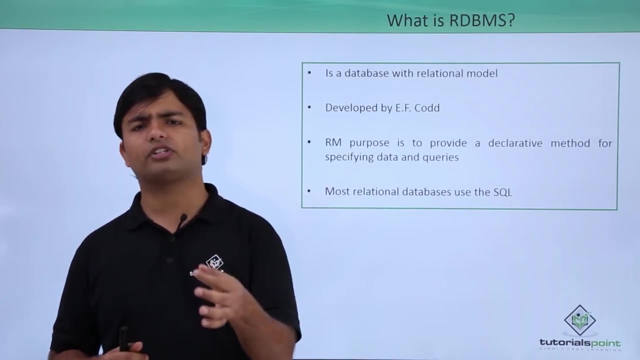 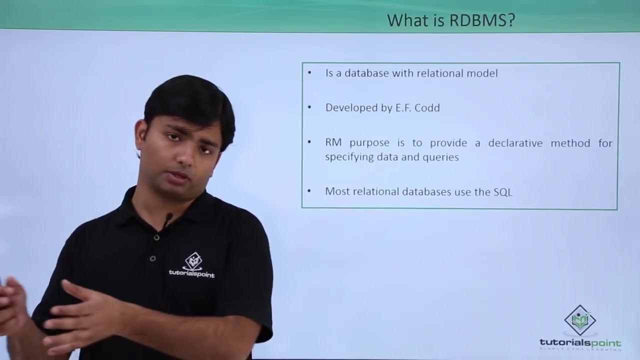 language is basically a standard language using which you can access almost all the RDBMS nowadays. yes, of course there will be a bit difference in each and every SQL. like maybe the function name will be different, something in Oracle will be having a different name in, maybe, MS SQL server. so 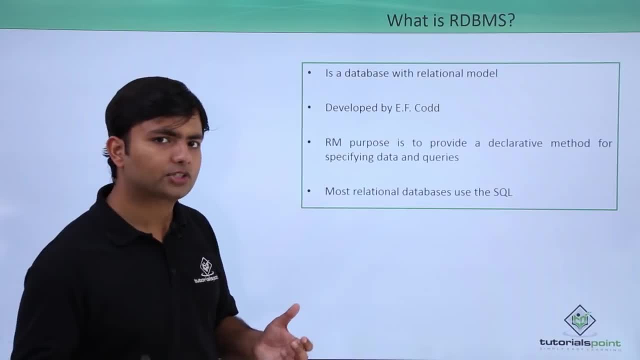 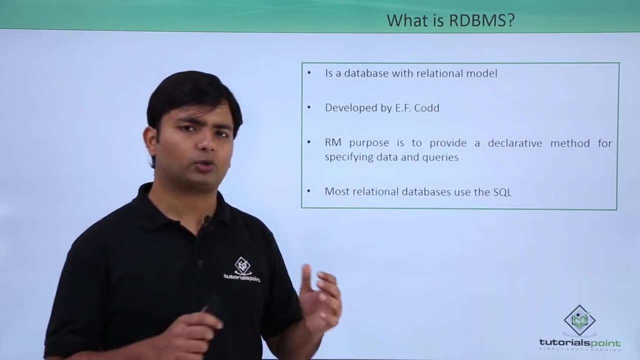 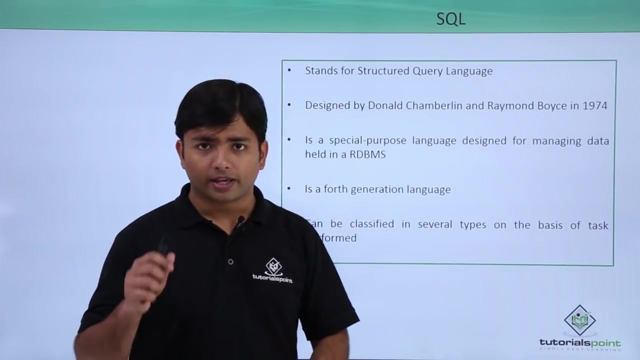 some basic changes will be there, but overall the language outline is going to be same and we are going to work with the SQL. so let's have a quick look what this SQL is all about. so, as I just said, SQL stands for structured query language. it is designed by Donald Chamberlain and Raymond Boyce in 1974, so initially it 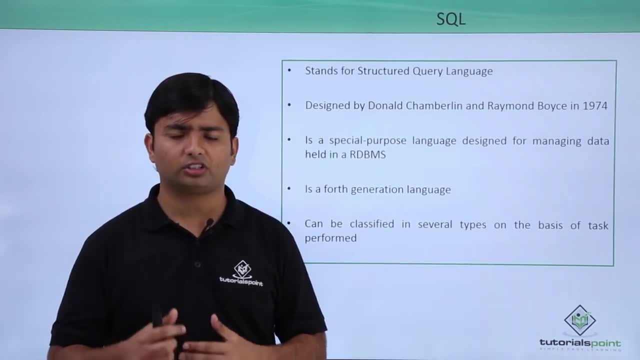 was used to retrieve the data from some of the databases. but since this language is a structured query language, it is designed by Donald Chamberlain and Raymond Boyce in 1974. so initially it was used to retrieve the data from some of the databases. but since this language 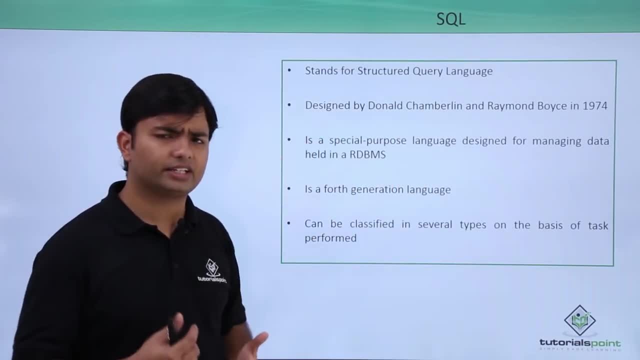 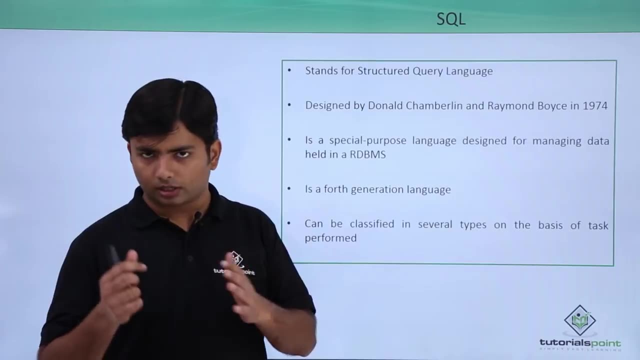 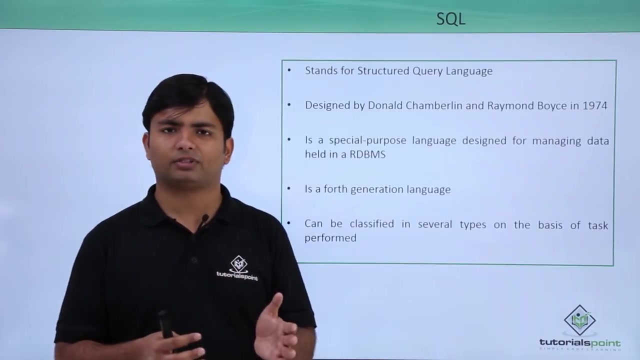 is very easy to learn. it is almost like an English language. so that's why it is categorized also in the fourth generation of language, fourth generation language, which is basically very much English type language, like we used to talk to each other. if I say something like delete from employees, so even if you are, 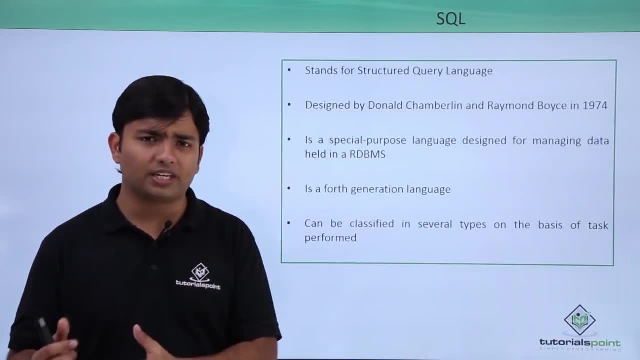 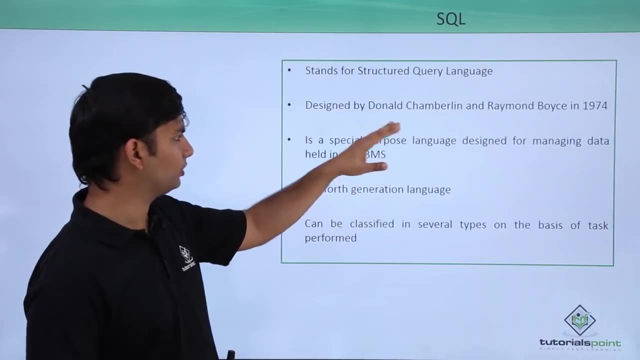 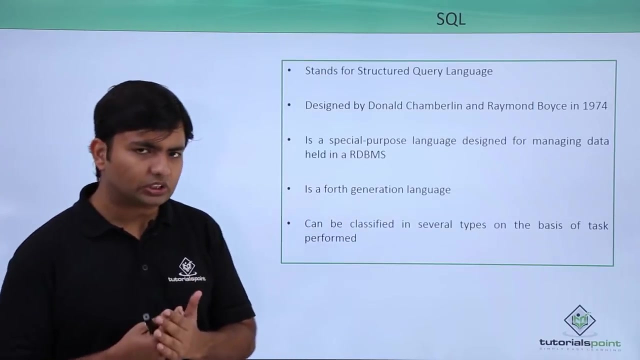 not family. with the SQL, you are getting actually what I mean. if I am saying delete, what does that mean? so this is as simple. so it's basic purpose is to. it's a special purpose language designed for managing data in our DBMS. using this SQL command, you can do different types of. 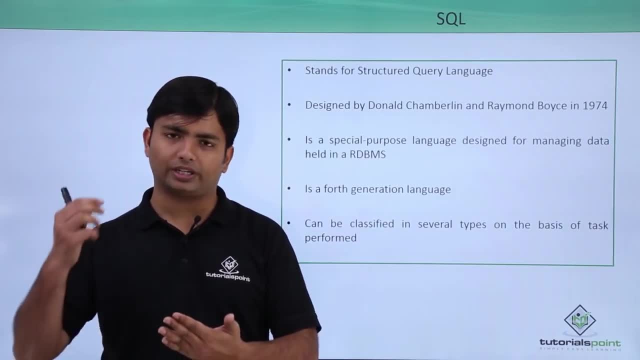 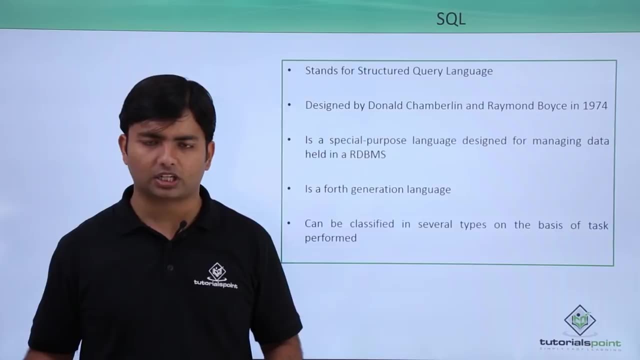 action like. you can create the new database object, you can insert the data, you can update the data, retrieve the data. you can delete the data. you can drop the structure of the table. you can do anything right, like allowing the user to get some privilege did revoking those. 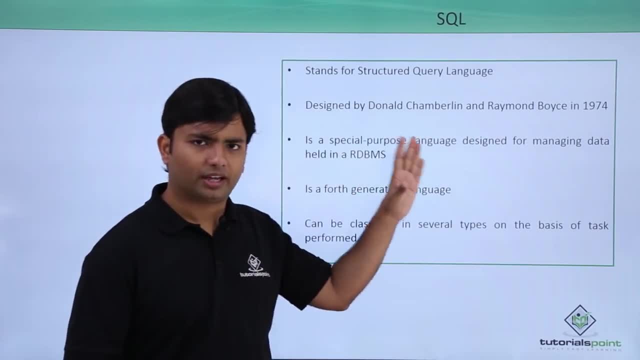 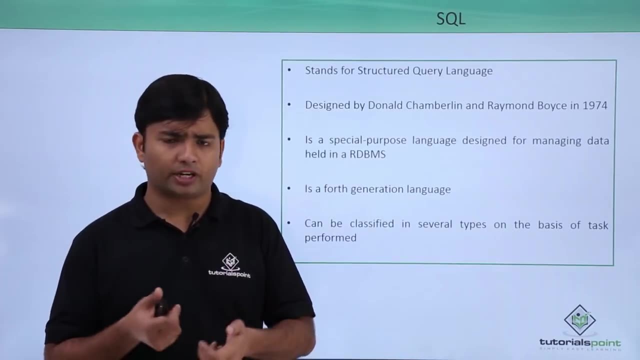 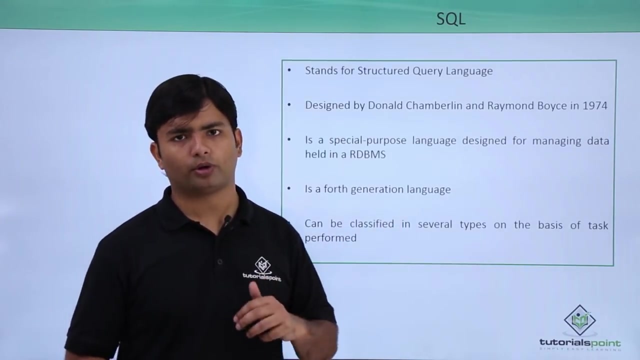 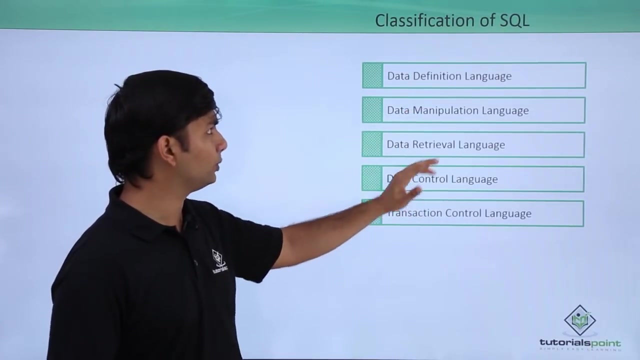 privileges. each and everything can be done using this SQL. that is structured query language, but, as I just listed, many of the tasks that we can do using SQL, we can actually categorize them as per their commands. so here we have the five major aspects of the SQL, five major classifications of the SQL. that is the 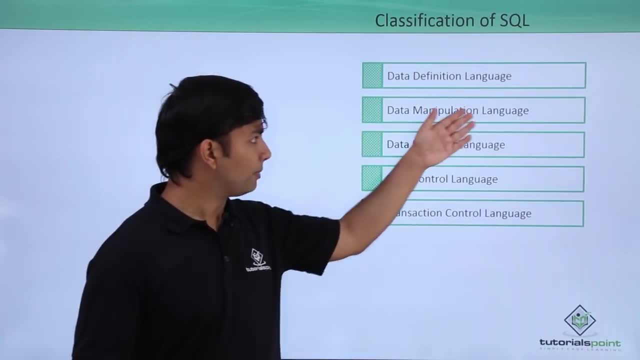 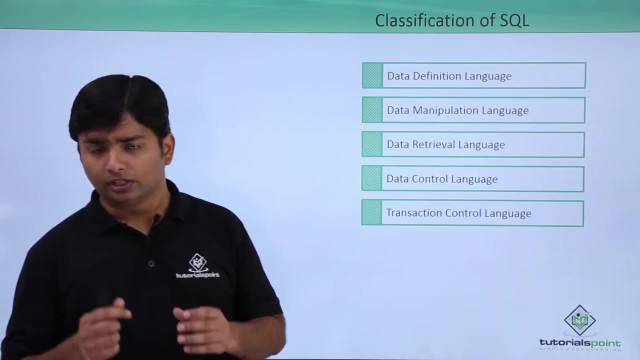 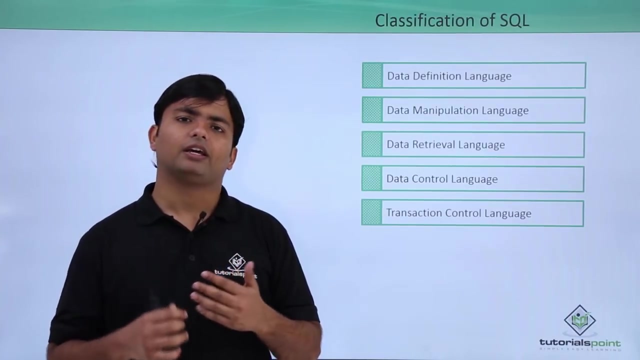 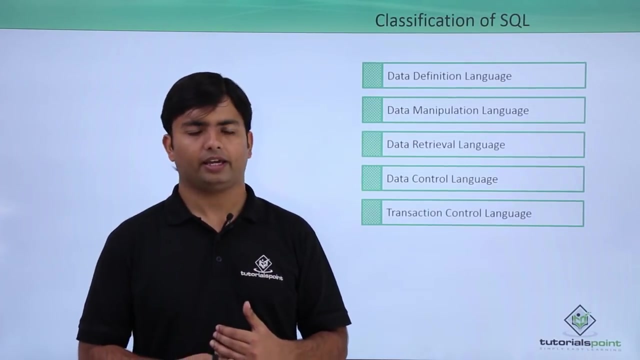 DDL, that is, data definition language, data manipulation language, data retrieval language, data control language and transaction control language. so let's have a basic idea of each data definition language means any SQL command which is actually used to define some database object, like if I am going to create a table, a view, an index or anything, I am adding a new object, I am 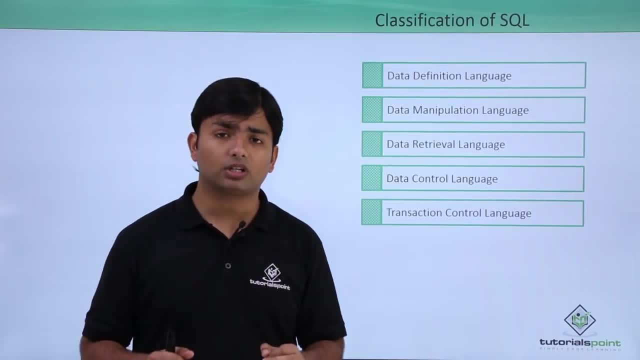 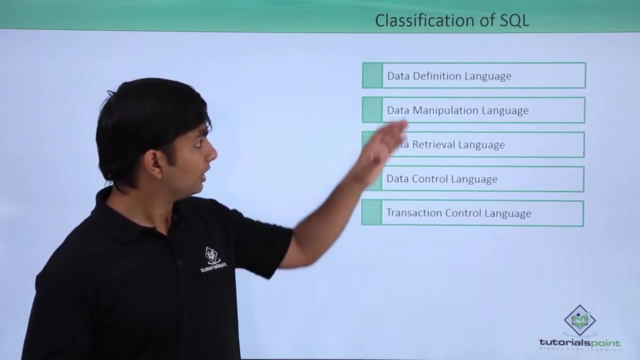 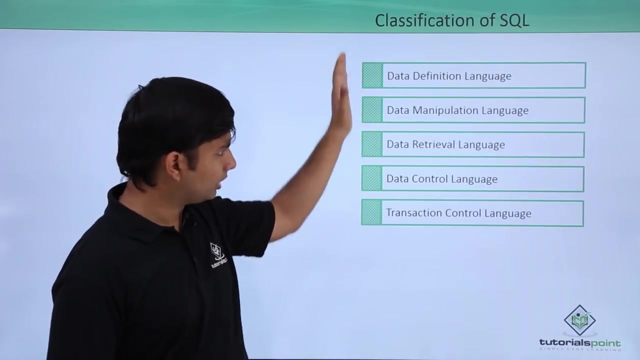 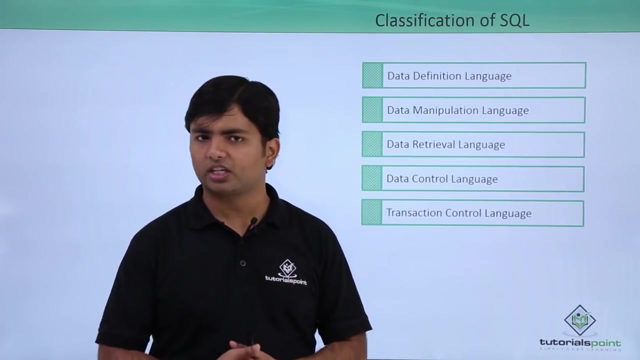 adding something new in the database. so if SQL command is affecting the structure or the information of database, I will categorize them in the data definition language you know. for the videos we will of course give a deeper look in each of these segments: data manipulation language. once you have created the table, now what you will have to insert some. 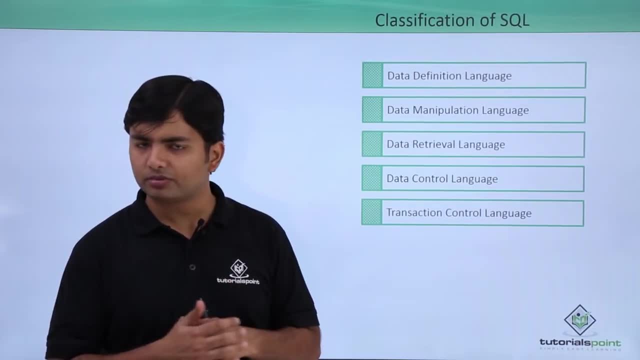 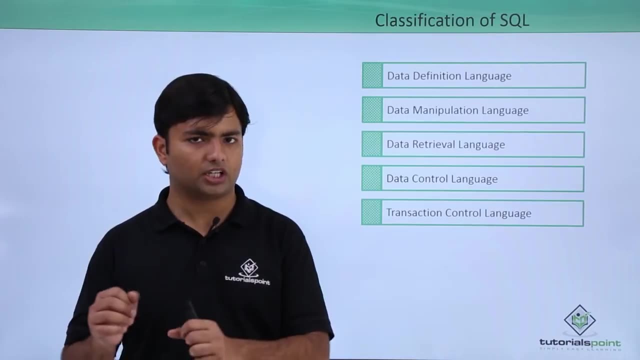 data. when you insert or manipulate some data, it doesn't affect the structure of database. but, yes, it does affect the structure of the table. like if I'm entering a new record, one new record is added in the table. if I'm updating, some data is gonna change. when I'm deleting, some rows are gonna removed. so this is. 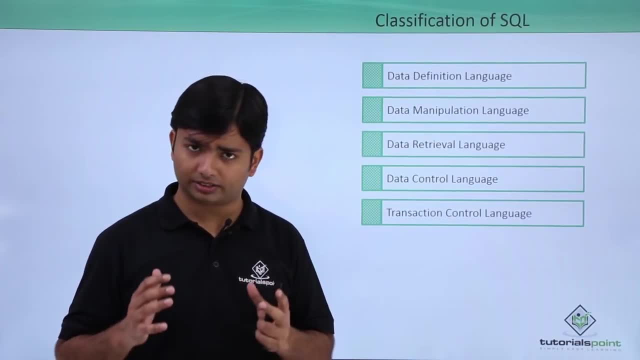 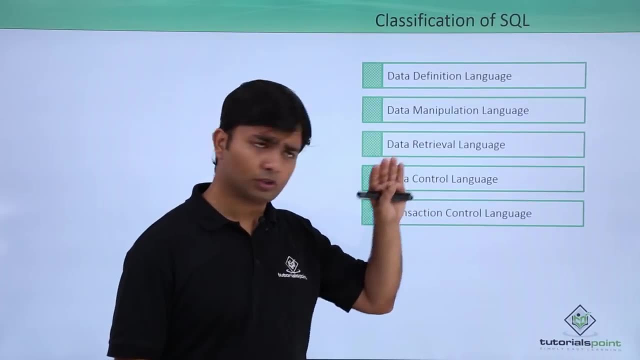 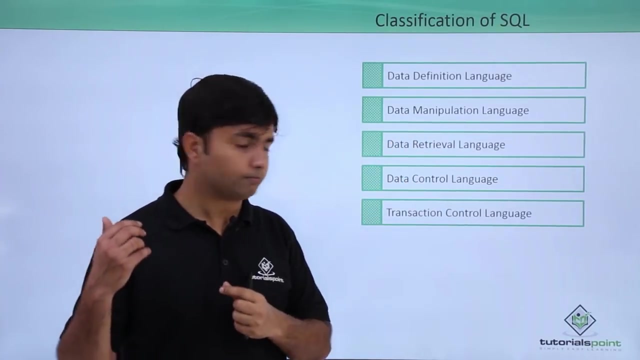 the data manipulation language. when any SQL statement will affect the data inside a table, I will categorize it inside the DML. now, once we have the data, we can start retrieving the data from the database and then we can start doing that. so that part will be deal with the data retrieval language or data. 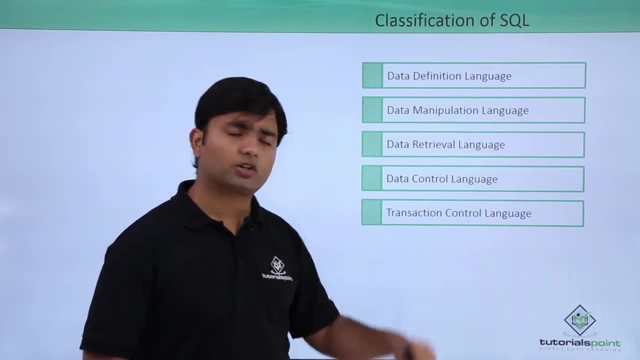 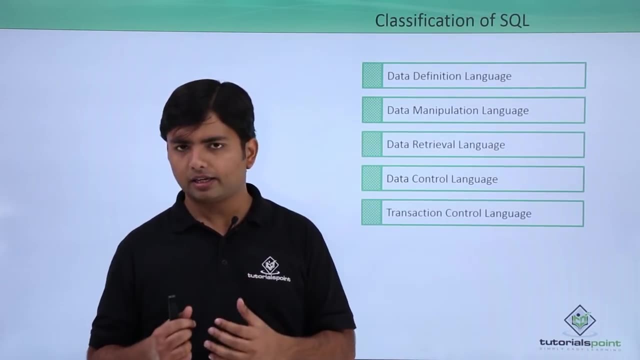 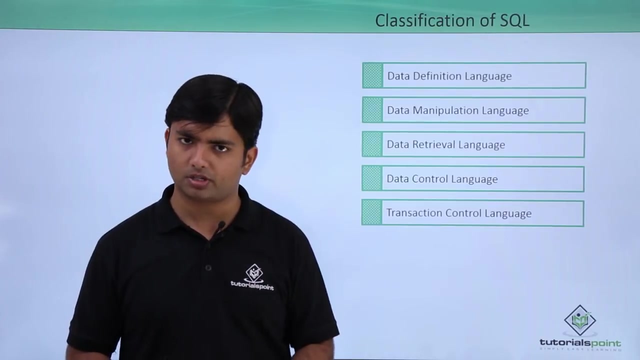 query language may be, in some data databases, data control language. this data control language actually deals with the accessibility, like if I'm working in a centralized database and there are number of users who can access the same database, I will have to specify the goal, for example. I should not say goal. 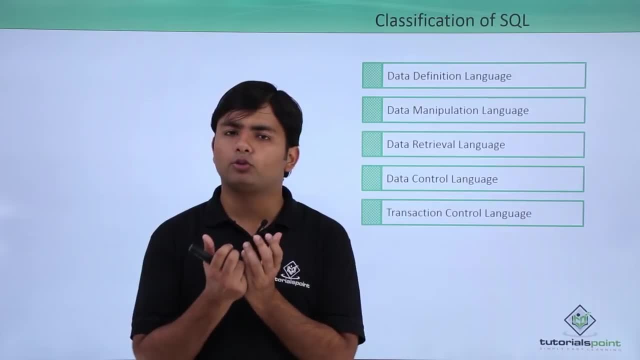 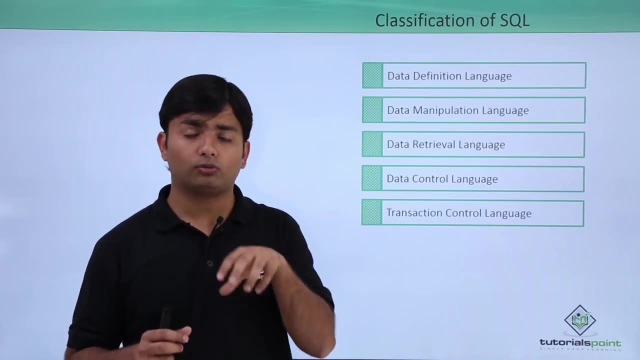 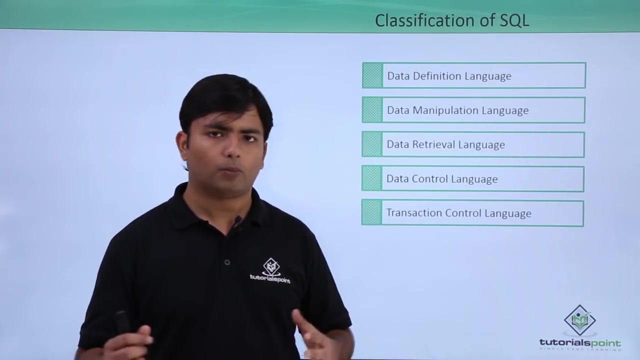 I should say roles. so when we have the different set of users and all are working in a centralized database, each user would be having a different role. means that role will be defining, like how much a user can access. even I can access a Google database through Gmail, but I can only check my mail, so somewhere 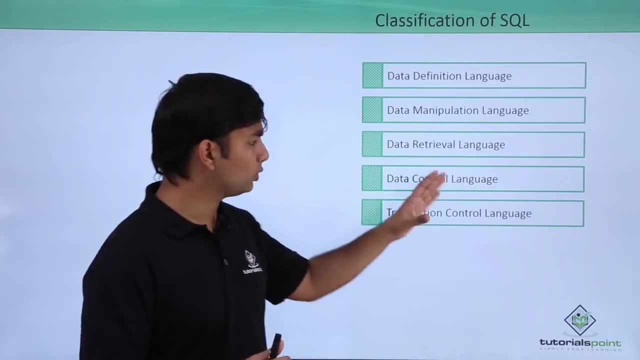 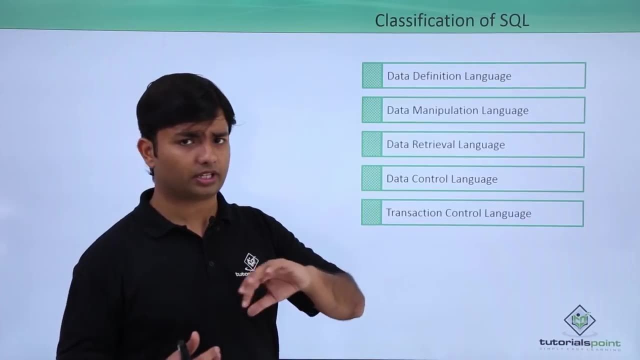 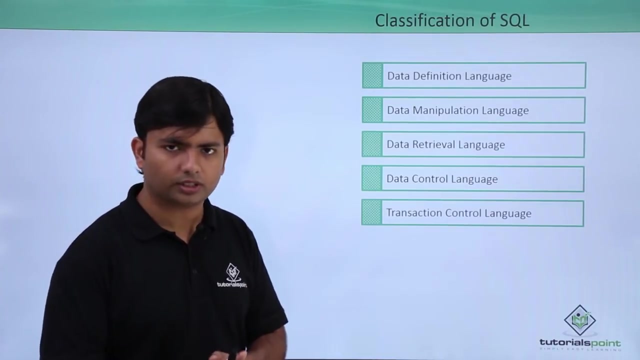 I am getting restriction, so that is what we can do right here. if there is some user who are in admin level, I will obviously allow them to create a table. they can access all the data from the table. but if there is some third user- third party user type user- is there, then I will only give some view of the 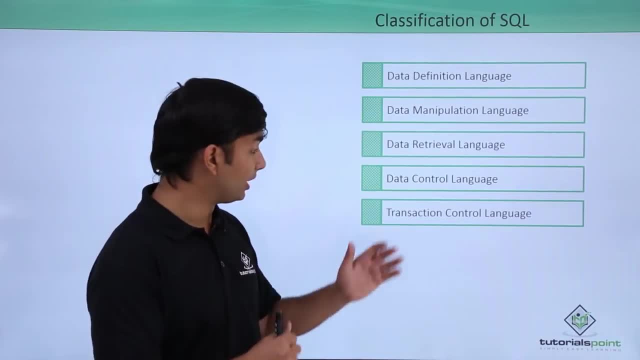 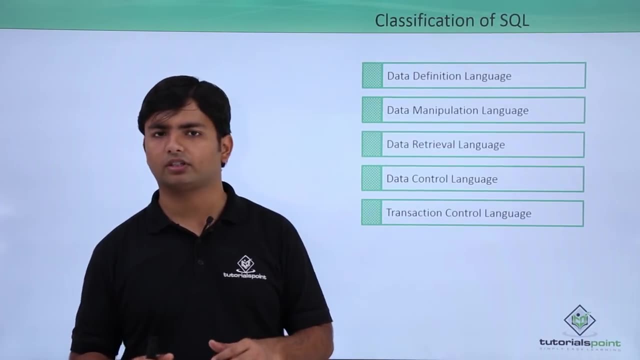 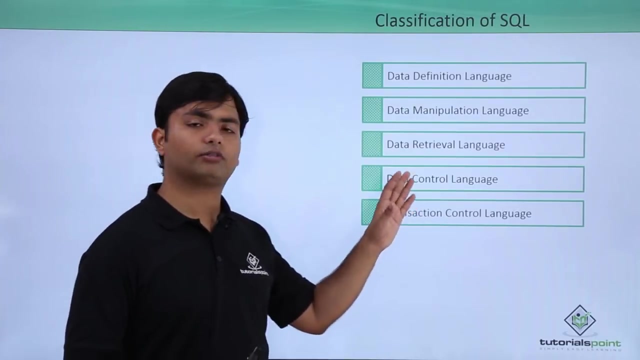 data means some particular things can be retrieved by some set of users. transaction control language. transaction control language simply means when I am executing a number of SQL statements all together, then I should take care of the transaction. maybe if I'm transferring some amount from my account to my friend's account, so there. 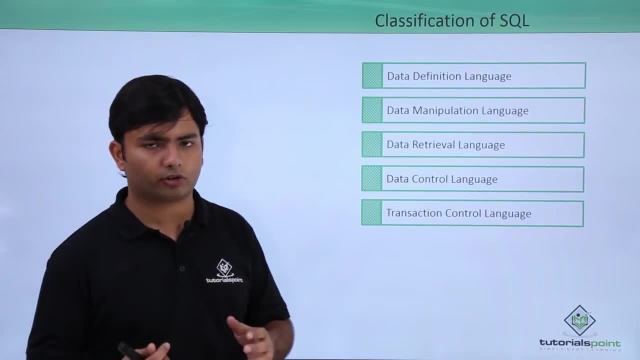 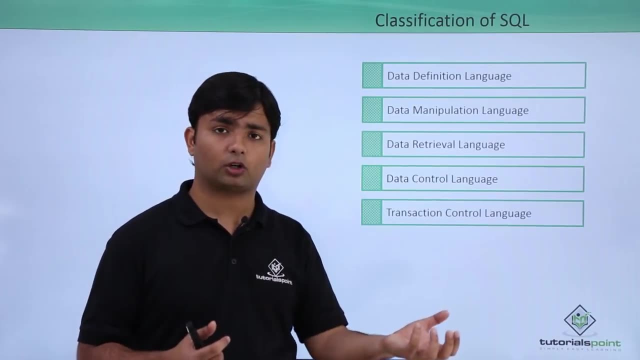 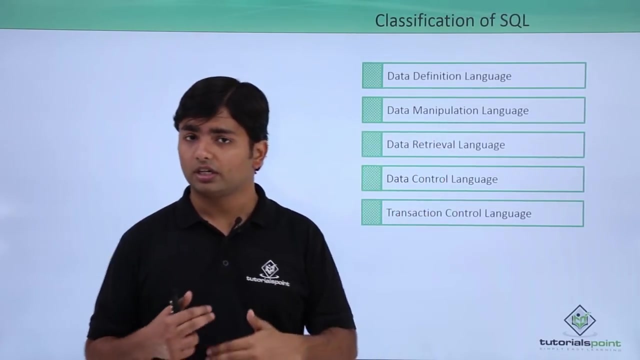 will be. a couple of SQL statements will be required. for example, first of all, I will update my account balance, will deduct some amount, then the amount of my friend's account will be added. so there are a couple of update statements or any particular statement. any DML statement is gonna execute, but this transaction. 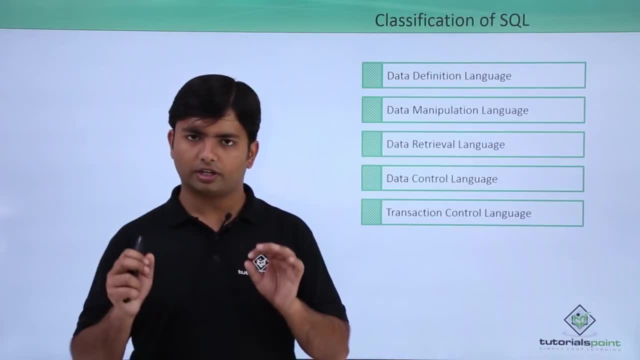 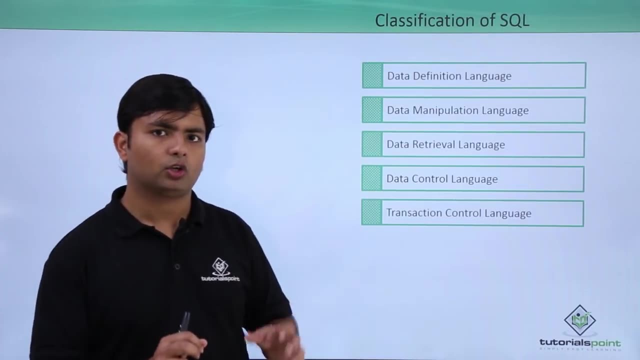 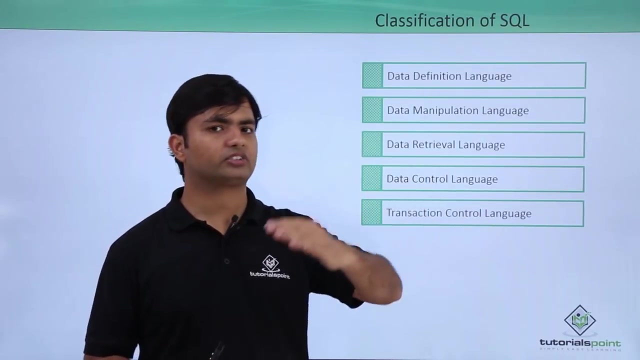 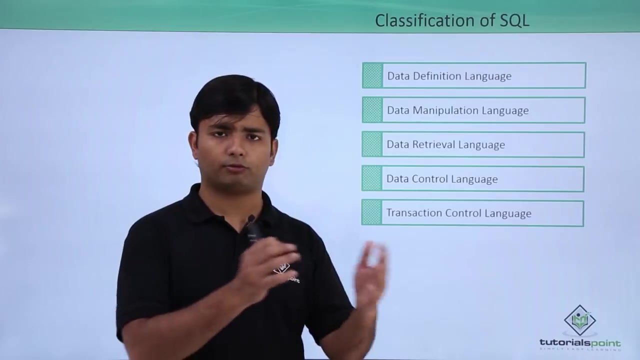 control language will ensure us, like if it is getting successful, both the commands or all the commands participating in a transaction will execute successfully. otherwise, if there is something wrong, obviously the whole transaction will be rolled back, not the half or some percentage of the transaction will be successful. either it will be fully successful or fully failed. 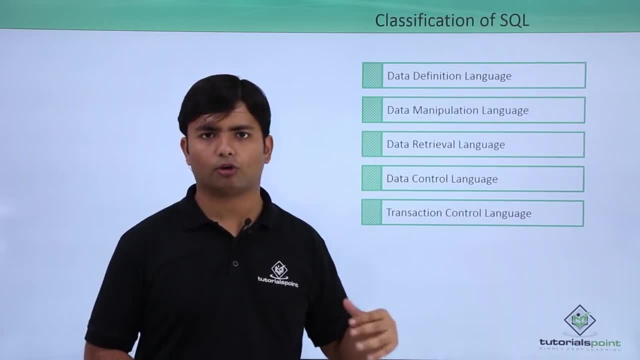 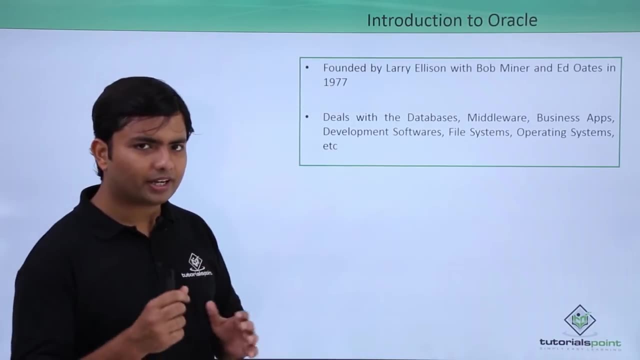 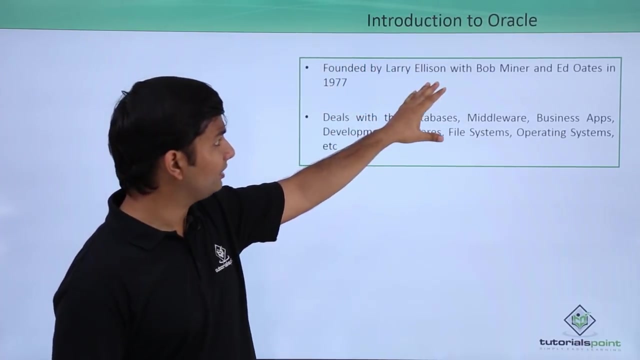 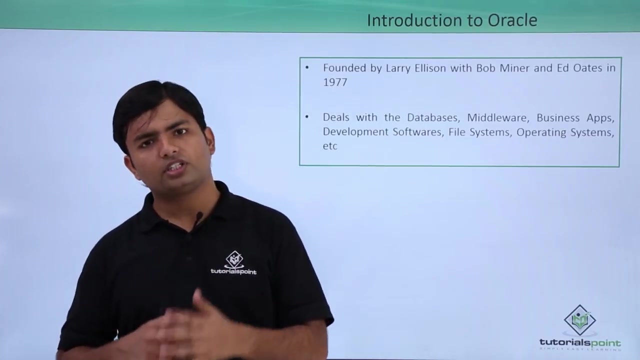 so these are the different classifications of SQL. now let's have an introduction of Oracle. as in the beginning, I told that nowadays it is a developed organization, but here the it is founded by Larry Ellison with Bob Miner and Ed Oates in 1977. basically, Oracle was initially just a product on. 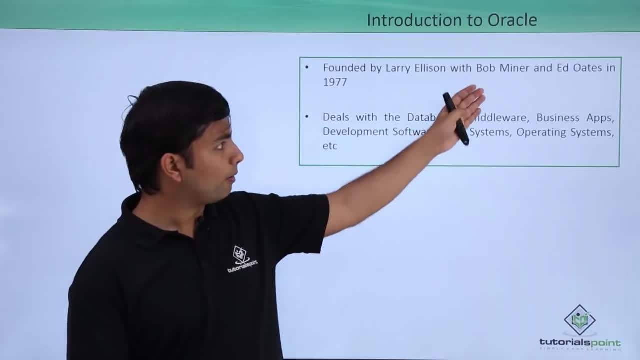 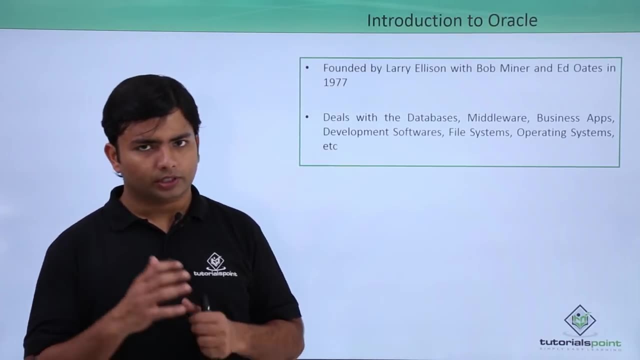 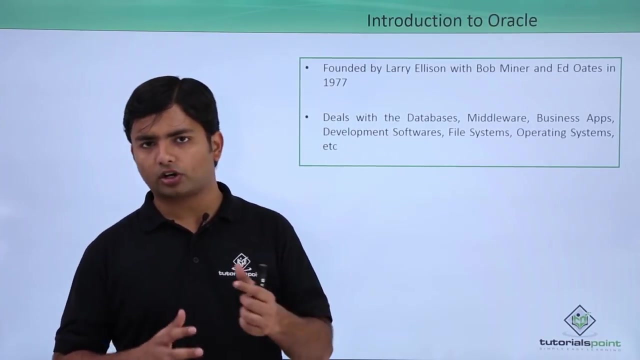 which Larry Ellison was working along with the Bob Miner and Ed Oates. basically, he was working on the RDBMS rules written by EF Codd and the product which he created. he named it Oracle. later he founded an organization with the same name and nowadays the